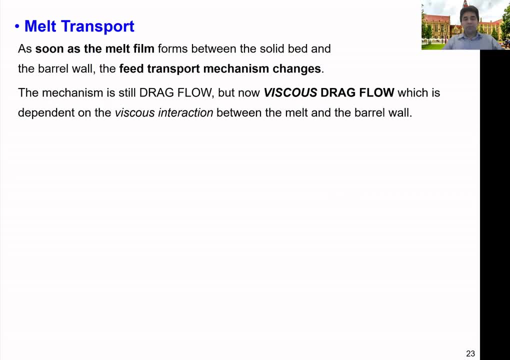 the barrel roll. So it is clear that in the solids conveying zone we had a pure drag flow, but now in the melting zone, as melt formation starts, so then the flow behavior changes from the drag flow to a viscous drag flow. So then, after melting takes place, what will happen is that? so then material. 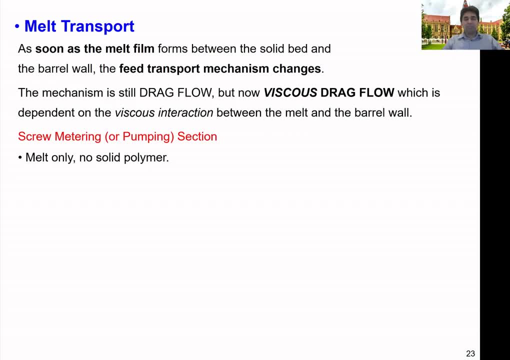 will pass into the pumping section, or we call it the metering section. Ideally, what we can expect is that within the metering zone there is no any solid material. There will be only molten material. so that is the idea, But sometimes there can be unmelted particles within the metering section. 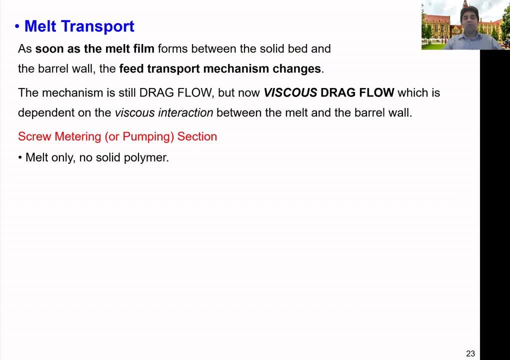 as well. so if you don't set up the the pressure, you can just go and put the material into the process settings accordingly, or if we choose inappropriate screw design or an extruder for particular material, so there will be some issues with having some unmelted particles within the 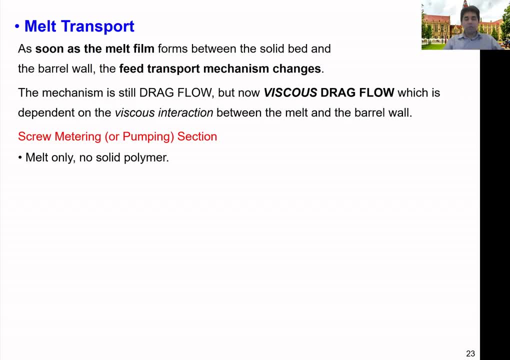 extruder output. actually so, but in the normal operation. so we don't expect any unmelted particle to be in the matron section, so it could have only the melt. so there is no solid polymer within the matron section. right here we are discussing about a single extruder. that means 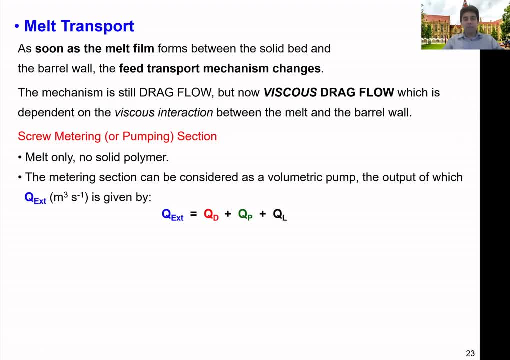 it's a continuous the process, actually, as long as you provide the material to the machine through the peat hopper, so there will be a continuous output. so the material will just undergo a few different processes. so initially they will be in the solids conveying zone and then absorb the heat. 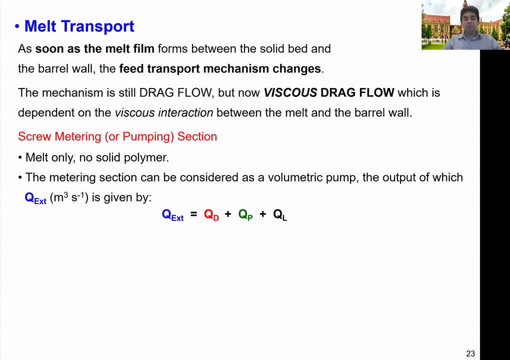 and then they'll become molten in the melting zone and then after that they'll be pushed into the matron zone. so then we can have the output, or we can just push the output to the die, so after getting that into the, the matron zone. so therefore the matron section of an extruder can be considered as a volumetric. 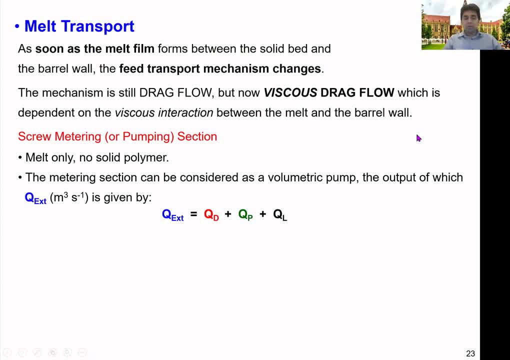 pump. so then we're going to get the output from the matron section so we can calculate the volumetric flow rate or the output from an extruder in cubic meters per second. so we can define it to be the qext. okay, so qext means the volumetric flow rate in terms of cubic meters per second. 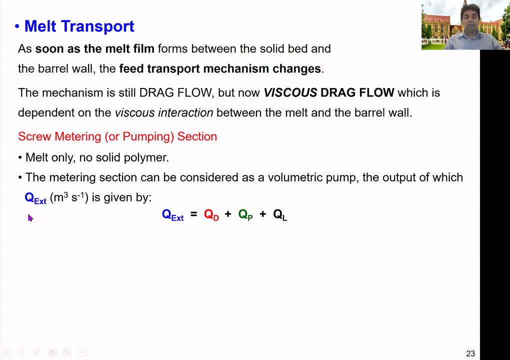 so that is the output from an extruder, as long as we provide a continuous speed material to the machine, so then we can maintain, uh, the relatively constant flow rate, uh, if you run the process uh within a constant processing speed, right? so then here we're going to look at how we can just provide an equation for 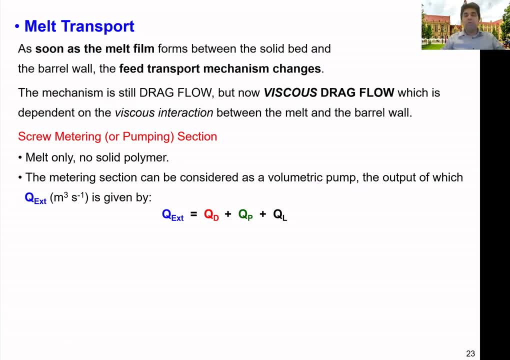 the volumetric flow rate of an extruder. okay, okay. so here we are going to look at how we can determine the volumetric flow rate of an extruder, or how we can provide an equation for an output from an extruder. so, by assuming that it's a continuous, uh the process, okay, so that means we're just going. 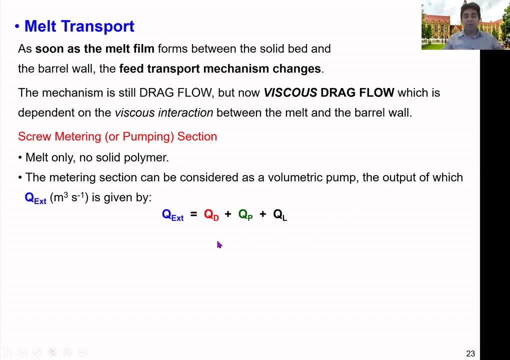 to feed the material continuously. so then we're going to have the volumetric flow rate of an extruder, can just develop an equation to get the output or the volumetric flow rate from an extruder, So it can be provided using this equation. actually, here We could see QEXT is equal to QD and QP plus. 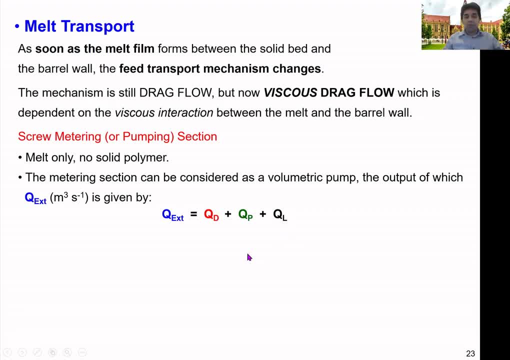 QL. So let's try to identify this term one by one. So, as I mentioned before, so this is the output rate in cubic meters per second right. So the QD represents the positive flow in the positive direction. okay, So it happens mainly due to the drag flow behavior. So we discussed: there's a 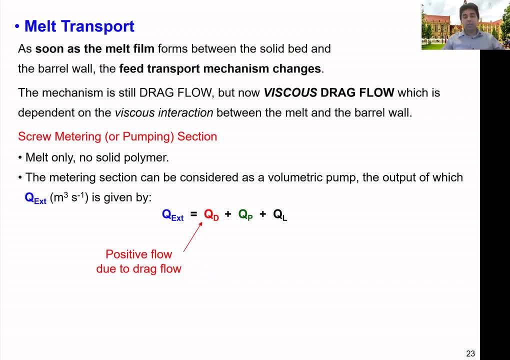 relative motion between the material and the rotating surfaces. So, due to that, so there'll be the positive flow which we can provide in terms of QD, which is we call the drag flow or the QD. right Here, the QP is known as the pressure flow. okay, It is a negative flow actually, So you can. 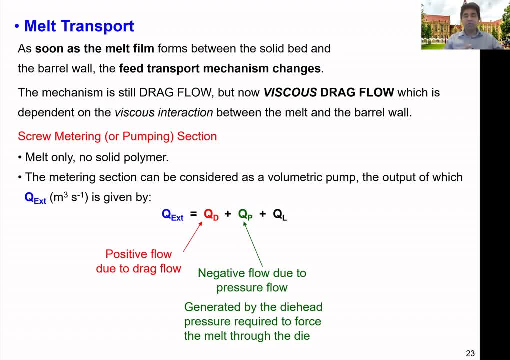 understand now. So we're just going to pick some of the die geometries or die units at the end of the extruder barrel. So due to that, so there'll be a pressure generation or equals the die head pressure. So normally if you just look at an extruder from solids, 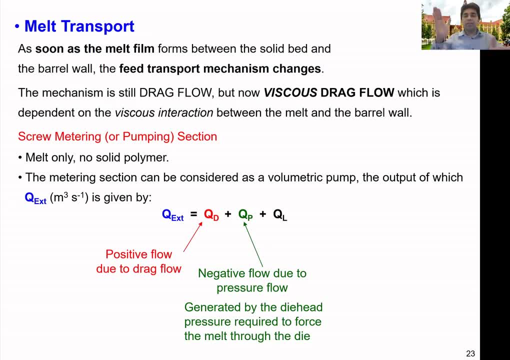 contained zone to the die. so the maximum the pressure would be at the die zone. okay, Because the metal is just pushing against the die. so to that end. So therefore there are the pressure generation, So the pressure profile from solids contained zone to the die will be increasing. 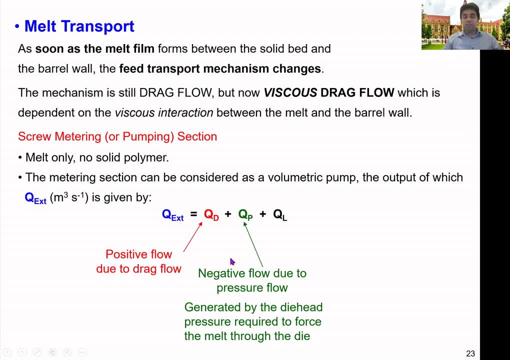 gradually. okay. So, therefore, this pressure just can create some negative flow, okay. So, which is represented by this QP? Here you can see that generated by the die head pressure required to force the melt through the die. okay, So we want to push the. 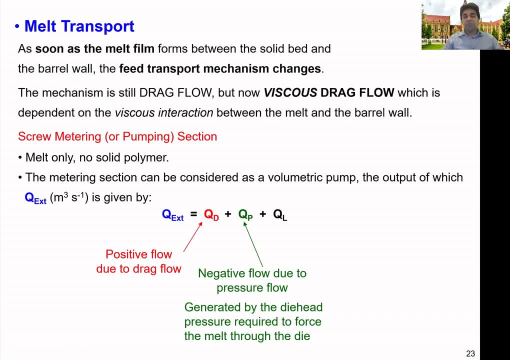 material through the die, but so that the pressure will just try to create some kind of disturbance to the inward motion or the forward motion of the material coming from the other zones of the extruder. okay, It is trying to hold the material due to the pressure generated at the end, okay. So 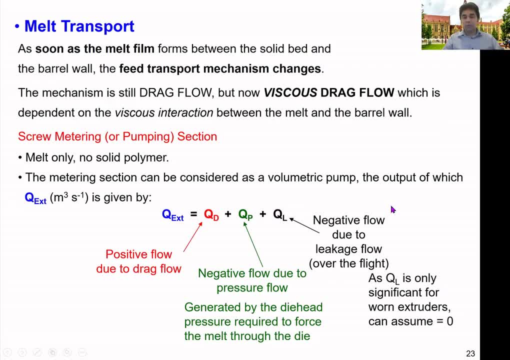 here QL represents a negative flow again, so we call it the leakage flow actually. So if you remember from the previous explanation that I made you for the Tadmo melting model, so I explained you that there's a slight clearance between the barrel surface and the top of each channel. 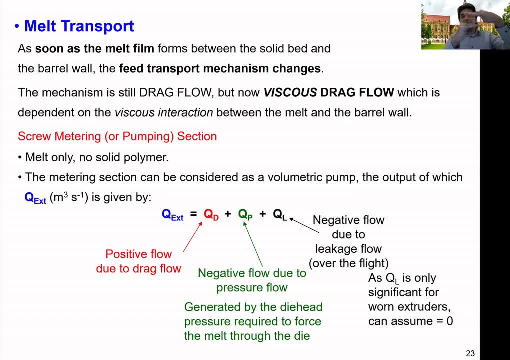 okay, So they are not just contacting each other. okay, The top of the scoop lights and the barrel surface: there's a clearance between them. okay, That clearance can just allow some material to go backward. okay, Not in the forward way or not in the way of the screw rotation. 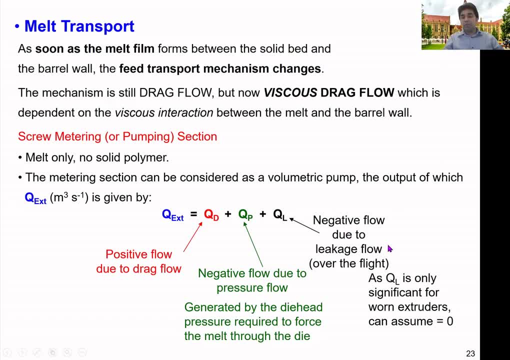 but in the opposite way, or the backward, over the plied. So therefore, so the QL is a negative flow, we call it a leakage flow. So this could happen through the clearance between the barrel surface and the top of the channel plied. okay, In fact, the QL term can be negligible for new screw designs. 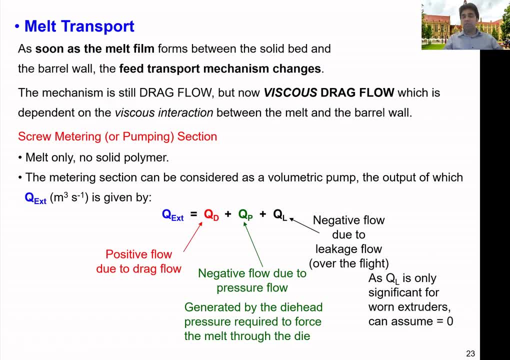 actually okay For new screws, the clearance between the top of the channel and the screw. the leakage flow is not that considerable for the new screws but with the time, with the wear and tear of the barrel and the screw, so then this could be a considerable flow, but for this unit. 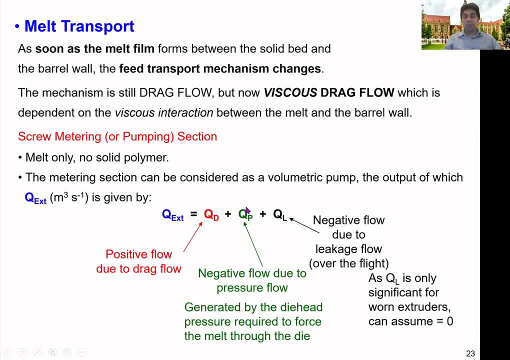 we can assume that QL is normally negligible compared to the other two. okay, So, as QL is only significant for worn extruders, we can assume here it to be zero. okay, So therefore we can assume that the extruder equation is given by in cubic meters per second. 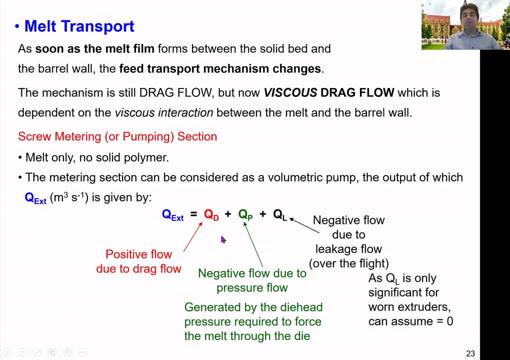 using these two terms, QD plus QP. So here QD is a positive flow and QP is a negative flow, and also QL is a negative flow as well, but in this case we can assume that the QL is negligible. 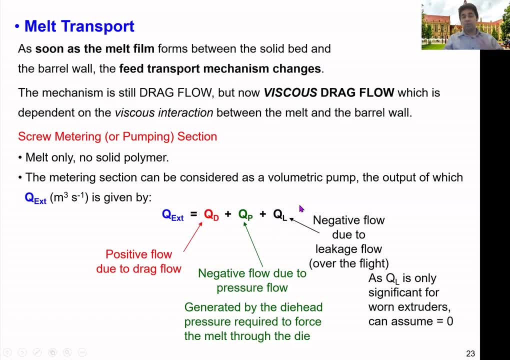 compared to these two terms. as long as the screw is in a good condition or the barrel is in good condition, okay. So this is what we call the extruder equation, or this is how we can calculate the output from an extruder. Here we can claim that for a given extruder, 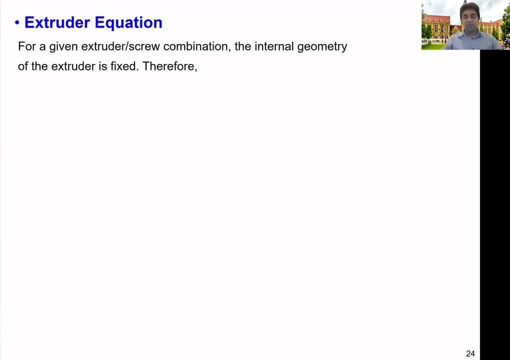 combination, the internal geometry of the extruder is fixed right. So actually we can just replace the screws in extruders, but for a given extruder screw combination the internal geometry of the extruder is fixed okay. Therefore we can define those terms QD and QP in detail. 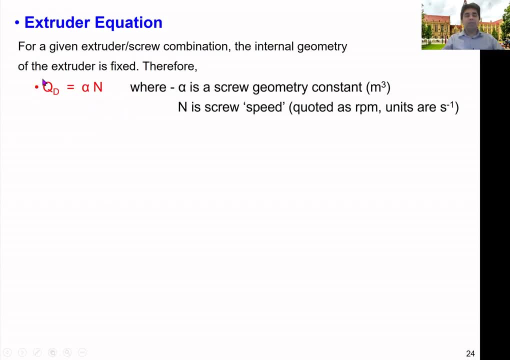 actually okay, For a normal extruder we can define the QD, which is the drag flow. okay, which is a positive flow, is equal to alpha times N. okay, So here alpha is a screw geometry constant. So this is a positive flow which is equal to alpha times N. okay, So here alpha is a screw geometry constant. 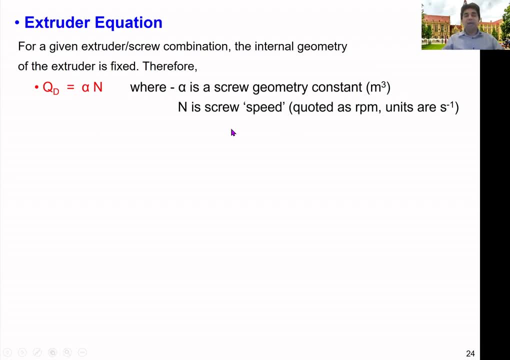 which is N- the cubic, the meters actually- and N is the screw speed, as is normally in rpm oh per seconds. right, So the N is something that you're going to set during the process operation. okay, So we can set the screw speed by setting the speed of the motor. okay, So a screw speed. 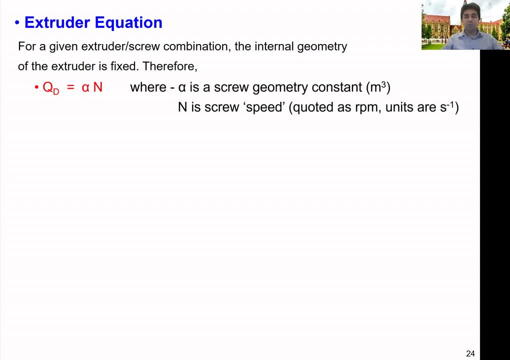 is one of the main process-controllable parameter for extrusion processes, right? So here how we can determine the alpha. is alpha can be determined based on the experiments, for example the N-screw extruder combination. okay, So then, so we can provide the pressure flow which is QP in. 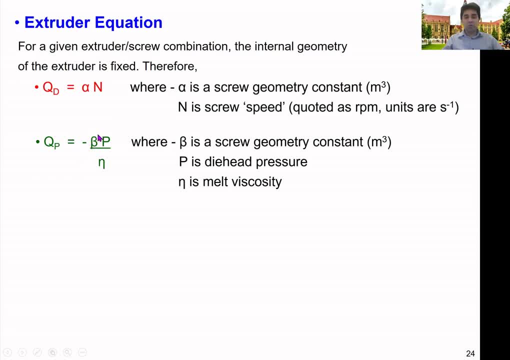 this format. okay. So beta is another screw geometry related constant, which is N cubic meters, and then the P is the die-head pressure, which could be in the Pascals or Omega Pascals, and eta is the viscosity of the melt, or the viscosity of the material being processed, And then, as I 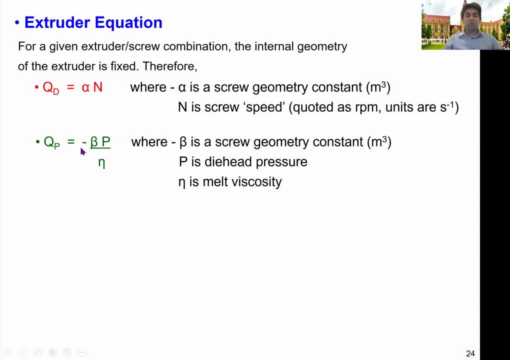 mentioned before. this is a negative flow. therefore, we have to just include the negative sign in front of this, the term actually okay. So then now we know how to just represent the QD and QP in terms of the process settings and also relating to the processing material-related. 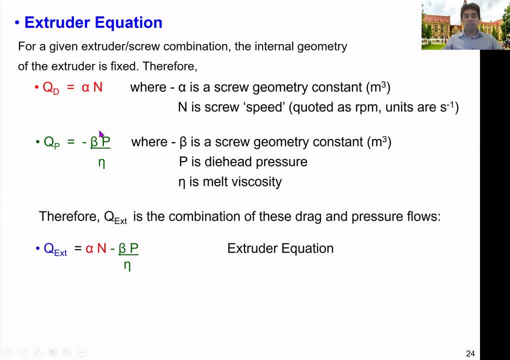 parameters right. So then, if you try to put them together, then so by just assuming that QL, a leakage flow, is equal to zero, so then we can just provide the output equation, or the volumetric output from an extruder can be given by: due to the drag and 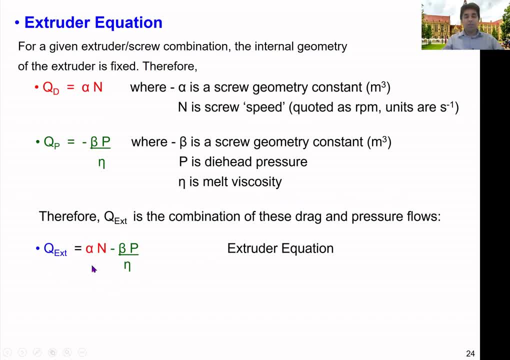 pressure flows in terms of this equation. now, QEXT, volumetric flow rate of an extruder is equal to alpha times N minus beta P over eta. So this is what we call the extruder equation. Remember that we can have the third term here as well, which is provided in QL. 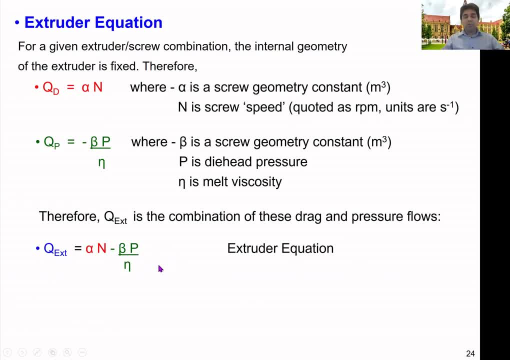 The QL can be dependent upon the clearance between the screw barrel wall and the top surface of the screw channel plied. Okay, as I mentioned before, the numerical values relating to the alpha beta, so which are the screw geometry-related constant, can be determined. 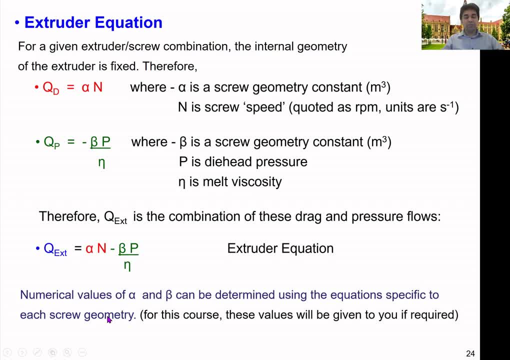 using the equations specific to the screw geometry, or they might be just determined based on the experimental observations as well, But for this course actually. so these values will be given to you if required. okay, Right, So now we know an equation. 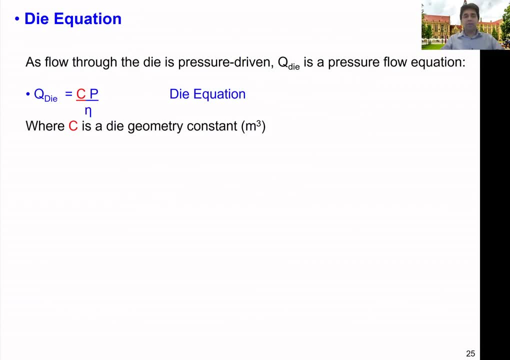 for the volumetric flow rate of an extruder, right? Okay, In the same way, we can define an equation for the die as well. okay, So we know that normally the flow flow through a die in extrusion is normally a pressure driven, okay, So therefore we can. 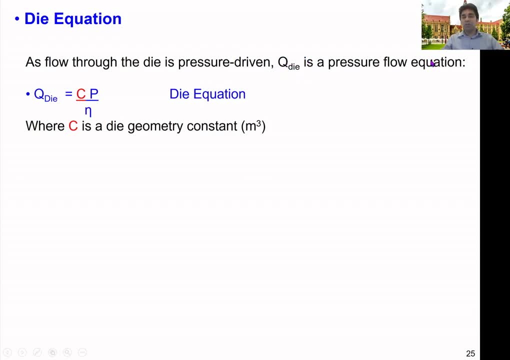 provide the Q die as a pressure flow equation. okay, So the Q die is the volumetric flow rate in cubic meters per second for a given die. actually, okay, Normally the flow through a die is a pressure driven flow, right? So most of the extruders can generate the required pressure to. 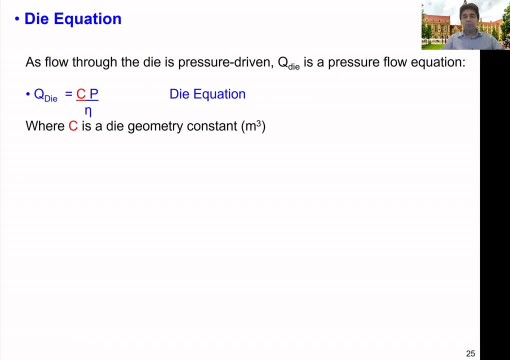 force the material through a die by itself, okay, So therefore there is no any other extra support is needed. as materials comes along there, the extruder barrel at the end, there could be enough pressure to force that material through a die, But in some occasions the pressure generated by 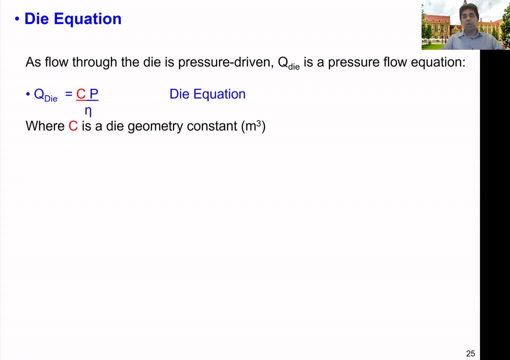 the extruder itself might not be required. So therefore we have to use some additional devices to generate the required pressure to force the material through a die. So in that type of situation we can use some devices like the screw pumps to generate the required pressure to force. 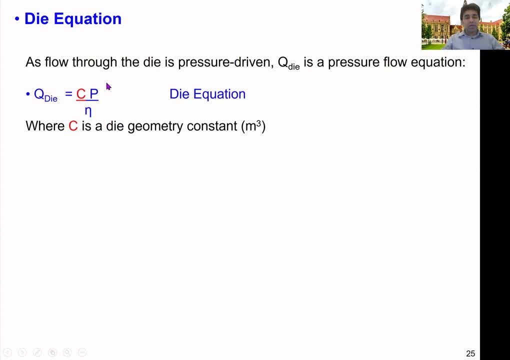 the material through the die. okay, Here, if you look at the die, you can see that the die is in cubic meters per second. okay, So that is, the volumetric flow rate through the die is equal to C. The C is also another constant, but it is a die geometry constant. 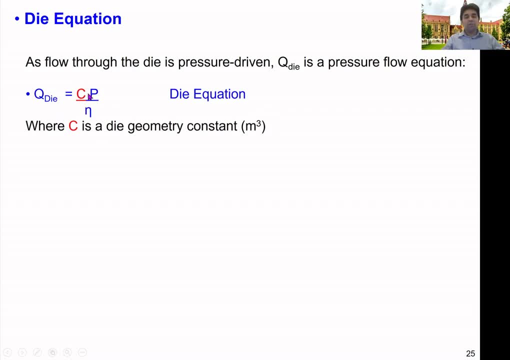 which is in cubic meters. okay, So then it's C times P, So that is the die head pressure, right And then. so this is what we call the eta, which is the viscosity of the melt, right. So therefore we can understand that volumetric flow rate through a die is dependent. 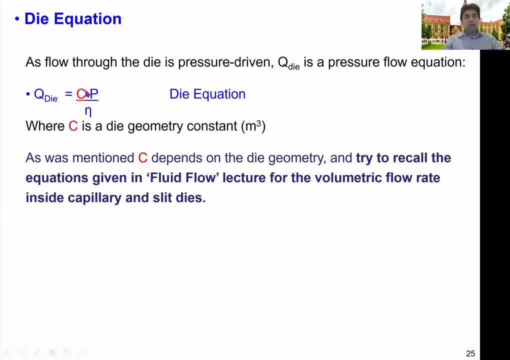 upon the die geometry, of course. okay, And then of course we can also use the die geometry and also the die head pressure and then also the melt viscosity right. The higher the viscosity of a given material, we need a higher pressure to force that material to a certain die geometry. 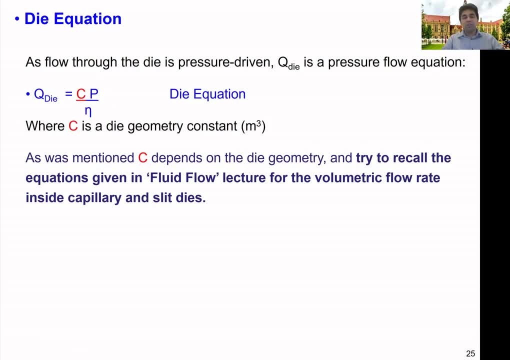 okay. So if you cannot generate the required amount of the pressure at the end of the extruder barrel, so then there will be some issues as we force the material through a die. So sometimes if you cannot generate the required amount of pressure, so we might not be able to. 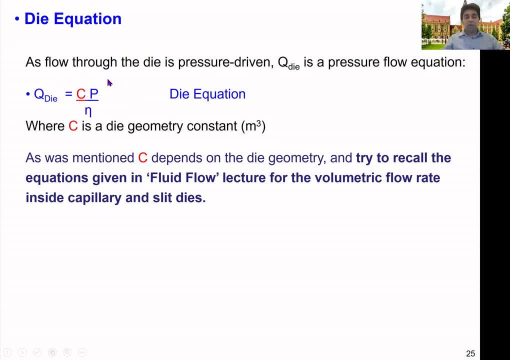 fill the mold smoothly in the proper way, So there could be some issues. So if you cannot generate the required amount of pressure at the end of the extruder barrel, so then there will be some defects with the manufactured product if you cannot generate the required pressure at the end. 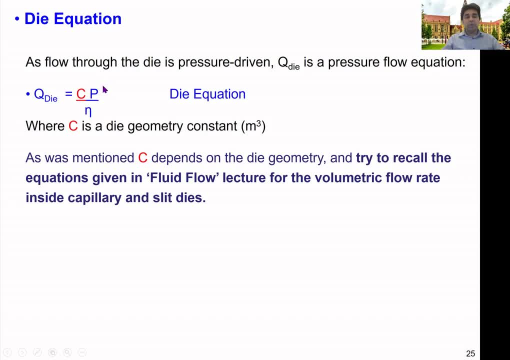 Therefore, it's really important to have some good idea about the required amount of pressure to force a certain material through a die. okay, So it depends on the die geometry, of course, actually, and also it depends on the material viscosity. okay, The higher the viscosity. 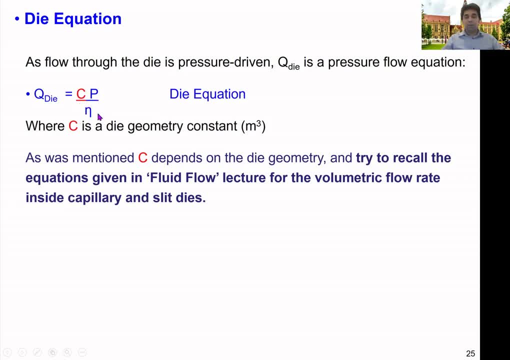 it's much harder for us to force the material through a die. okay, So, but here what we can do is mainly so we can select the proper set temperature at the die. So then, that means, in that way we can control the viscosity and also, if you want, to control the 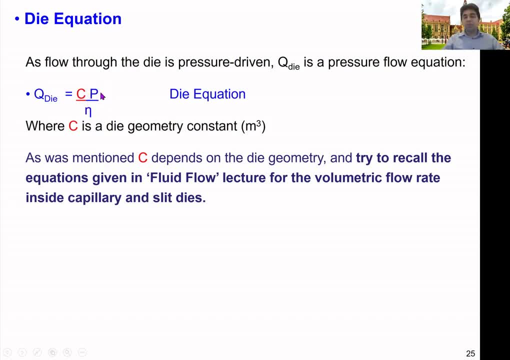 pressure, the one possible thing is to just control the squeeze speed, right? So then, these are not something that we can control directly, but we can control them indirectly. The viscosity of the material can be controlled based on the squeeze speed, and also set. 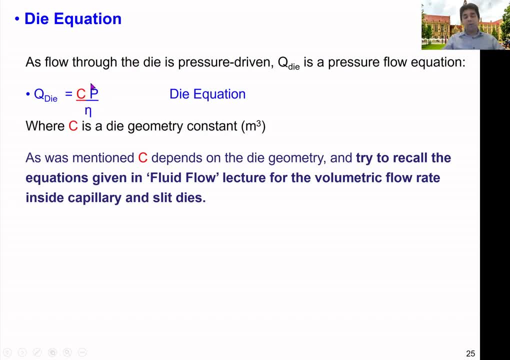 temperatures and the pressure also can be controlled based on the set temperatures and the squeeze speed. but the main effect can be just introduced: Increase in or decrease in the squeeze speed. okay, So hope it is clear. So that is what we. 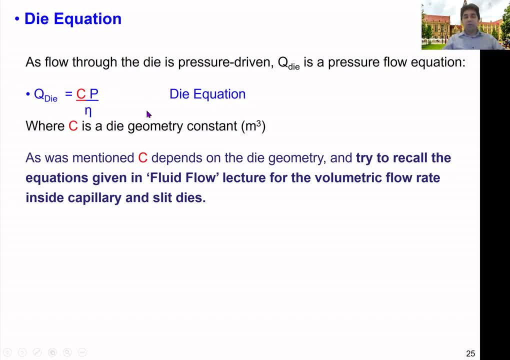 call as the die equation for a single squeeze through them right. So now we can quickly look at how we can determine this constant C, which is a geometry-related constant right. If you try to recall, in the lesson one we discussed the flow within capillary and 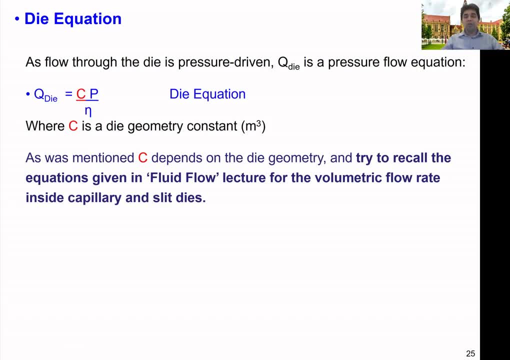 slit channels. okay, So we just developed some equation for the volumetric flow rate within capillary and slit dies. So then, if you try to recall those now, So this was the capillary die equation, or the volumetric flow rate through. 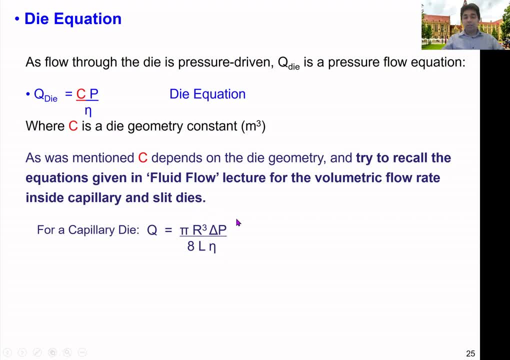 a capillary die. So this is for a Newtonian, the fluid actually. okay, So we call this Poisson equation for a capillary die. So that will provide the volumetric flow rate through that type of die in cubic meters per second. So here pi and then r to the power. 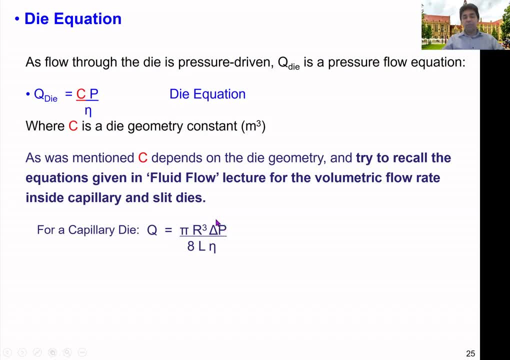 three is the. this r is the radius and this is the delta, p, that is the pressure difference. So this is: l is the channel length, and then eta is the material viscosity, right? So then, if you remember now? so look at these. 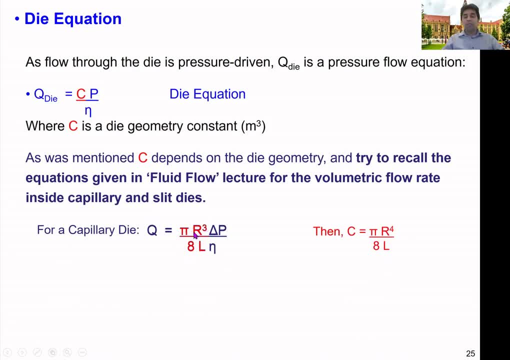 the four terms here: Pi is a constant for a given channel, radius is a constant and also length is a constant for a given channel. okay, So these two are related to the geometry right, And delta p is just something related to the process settings actually, and also. 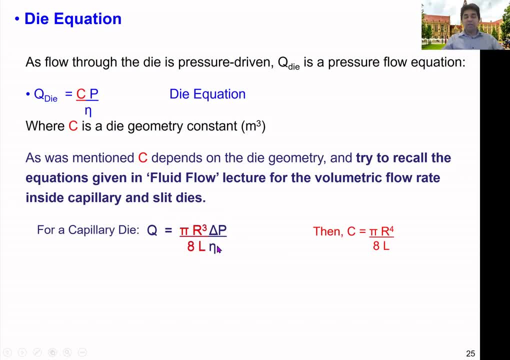 it's related to the geometry as well, actually. So the eta is a material parameter, okay. So therefore, you could say that This is the c. now, If you try to compare this equation and this equation here now, we could see that the delta p or the p here and viscosity, and then here p over l, is the same. 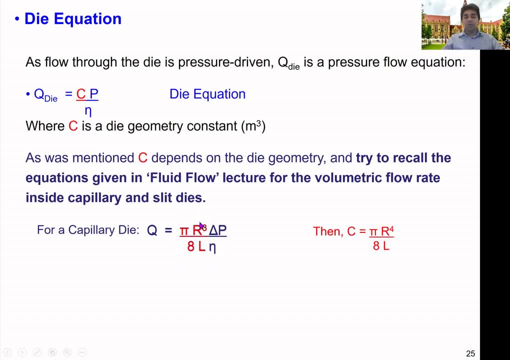 thing. So they are for a capillary die. So the c is this okay. So then you can recognize that the c, or the geometry constant or the die geometry constant for a capillary die, is this one here. Therefore, the die geometry constant for a capillary die can be given by this equation. 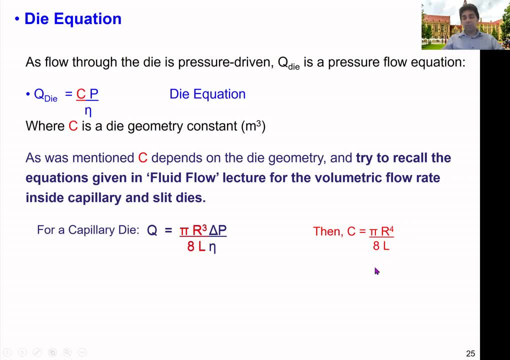 which is pi times radius to the power four divided by eight times l. okay. In the same way, if you try to compare this equation with the equation provided for the slit die. So in our lesson one. okay, remember that this equation 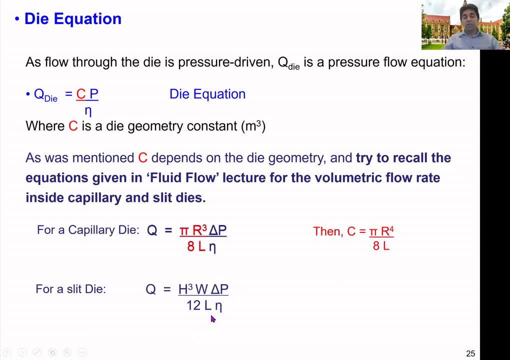 again for a Newtonian fluid. okay, Right here you can again recognize that delta p over eta term, or the pressure divided by eta viscosity. So then this part should be the related the constant for a slit die, Therefore for a slit die, so we can recognize. 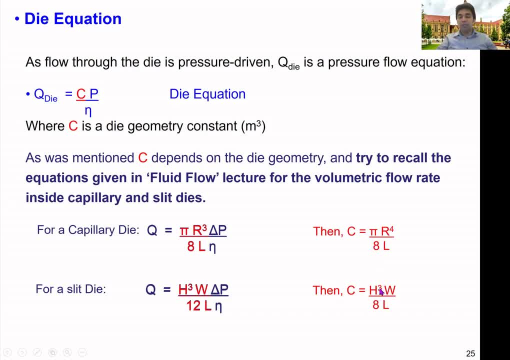 the constant is the h to the power three times w divided by eight l. okay, So here h is the channel height, okay, So then it could be a channel like this, So h could be this: okay, And then. 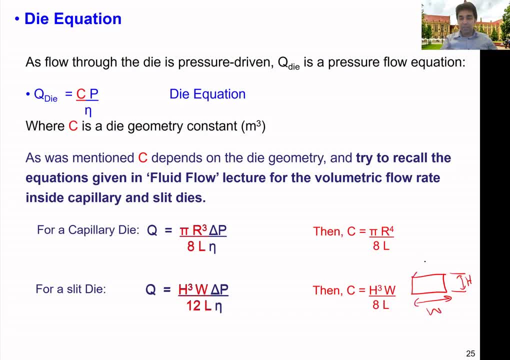 the w is the width, okay, And then l is the length of the channel. like this: okay For this one, for the capillary die now. so then r is the radius and then l is the length of the channel. 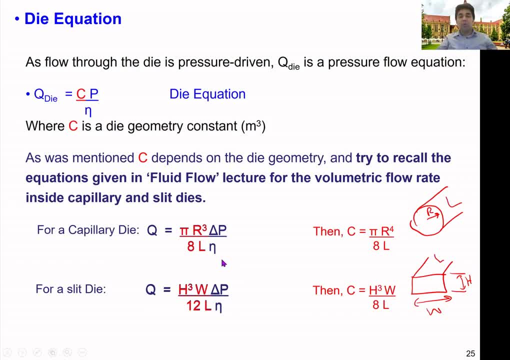 in this way. right, Therefore, it is quite simple. right, So we can recognize that delta p over eta term. okay, So this is quite easy for us to recognize the die constant or the die geometry constant for a capillary die and a slit die. of course, we have discussed these equations in the 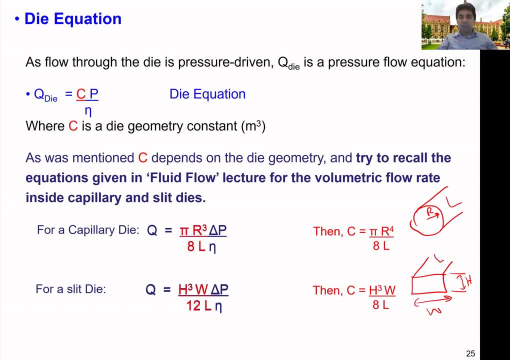 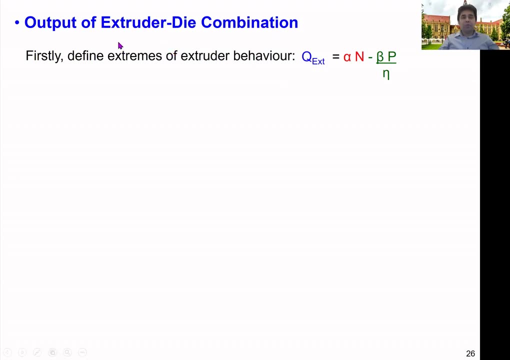 lesson number one. So now we can understand why we discussed before the heat transfer behavior and fluid flow behavior relating to this unit. So those are really directly related with the material processing applications. okay, So then let's try to understand the output of. 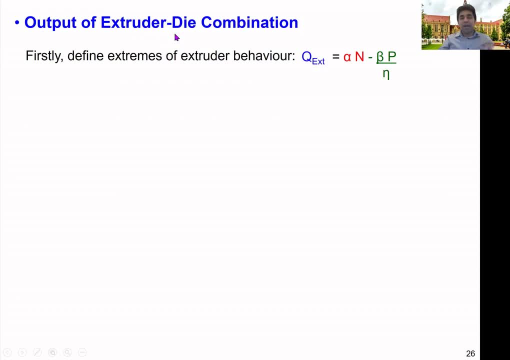 extruder-die combination actually. So we have an extruder and we have an extruder, and we have an extruder, and then at the end we have to connect it with a die. okay, So this pressure. 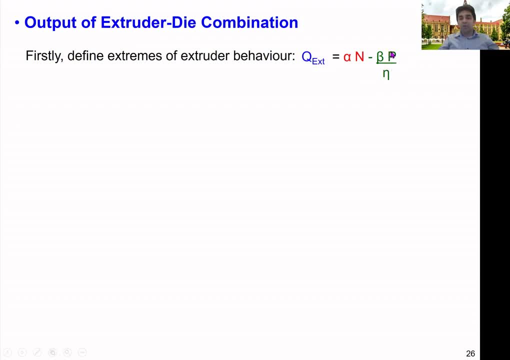 we call the die head pressure okay, So that pressure is generated because of the die attached to the machine at the end. So therefore, some of these terms should depend on the die geometry attached to the machine as well. The first situation that we can discuss is an open discharge. 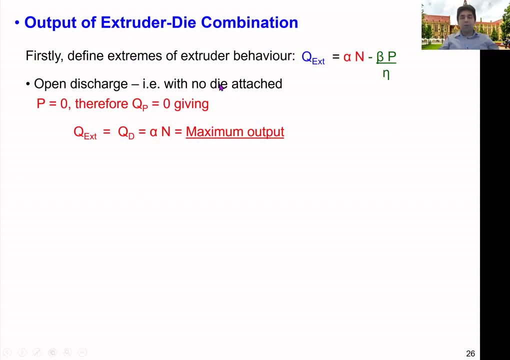 That is a situation with no die attached to an extruder. okay, So in that case we could say: P is equal to zero because there is no die attached, So there is no die head pressure. then okay, So therefore the QP, or the pressure flow, is going to be zero, right? So therefore, 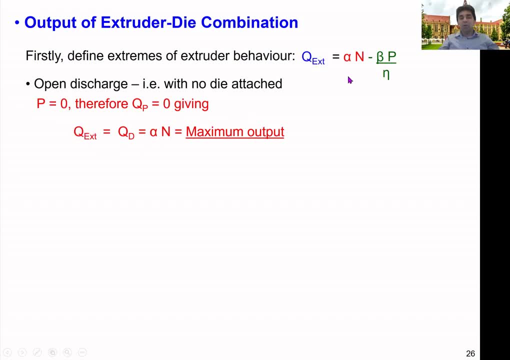 we can provide, then the output of the extruder just purely based on the drag flow, actually QD. So therefore QEXT is equal to QD, or the drag flow which is alpha N, So that is the maximum possible output that we can generate from an extruder. So that means without a die. 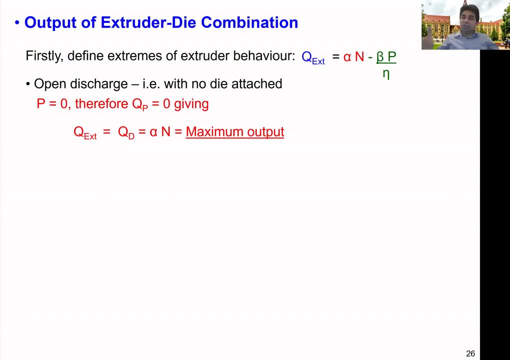 you can understand that there is no any. the resistance to the material flow: okay, There is no obstacle at the end, So there is no die attached. So therefore the pressure generated at the end is really minimal. So therefore, 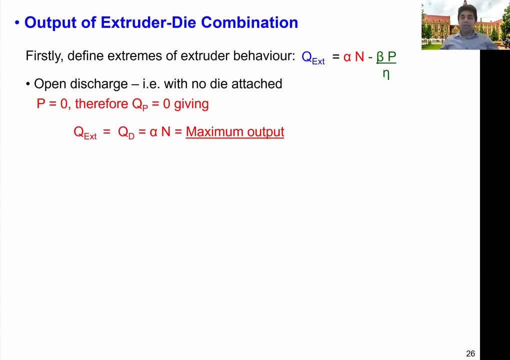 we can have the maximum possible output without a die at the end of an extruder, okay, So open discharge is the maximum possible output that we can have from an extruder for a given speed. okay, The second situation that we can discuss is a closed discharge. okay, So. 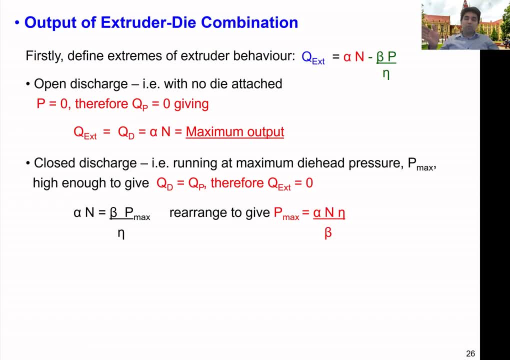 if we don't get confused here, that does not mean that we're going to close the end of the extruder barrel, okay, So we can't do that while extruder has been running. So if you do that, it could. 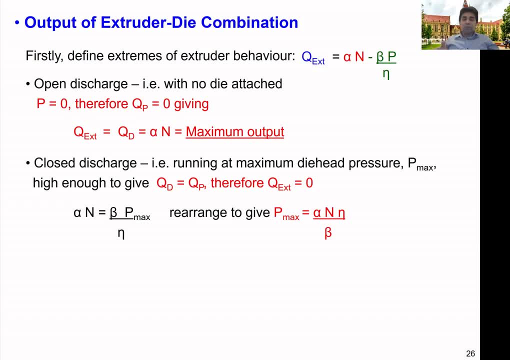 create some accidents, actually, okay. So that means if you try to close the extruder barrel while it has been running, so it could just generate the enormous pressure at the end of the barrel, So sometimes it could cause to expose the extruder as well. okay, But here what is the 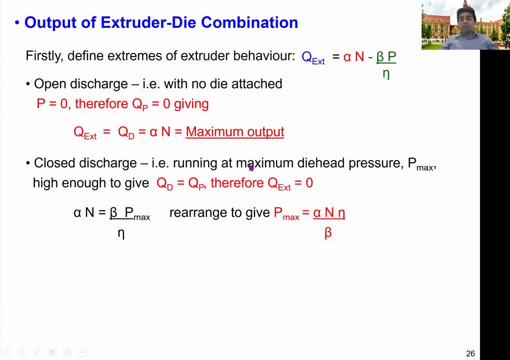 meaning of a closed discharge is that they're running at maximum possible diehead pressure. So in that way we can get the maximum pressure, or the maximum diehead pressure we call Pmax, So to get the maximum possible pressure. so we can just assume that QEXT is equal to zero. But okay, this is not realistic, okay, So 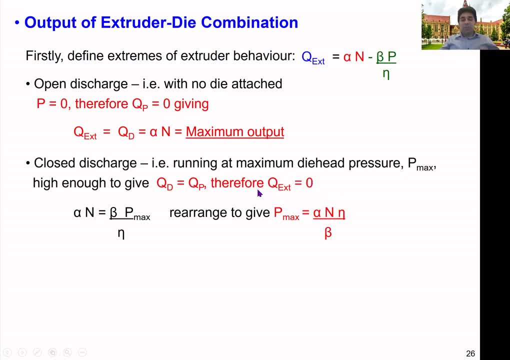 don't try to run an extruder by closing the end, right. So here the idea is: let's say the QEXT is zero, then So that means we can say that QD is equal to QP, The drag flow is equal to pressure. 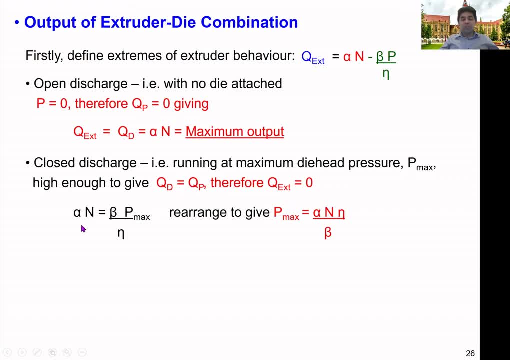 flow right. So in that way now. so if you try to put the terms related to them, the QD is equal to alpha N And then equal to beta Pmax over eta. So in that situation, when QEXT is equal to zero, we call. 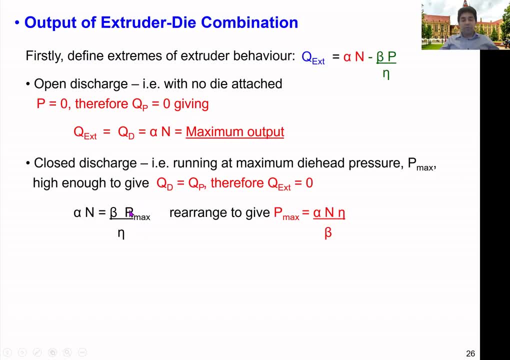 that this P is the Pmax, That is, the maximum possible diehead pressure. So if we try to rearrange the equation so that we can have the Pmax, the maximum possible diehead pressure is equal to alpha times, screw speed times. viscosity of the material divided by beta. okay, So that 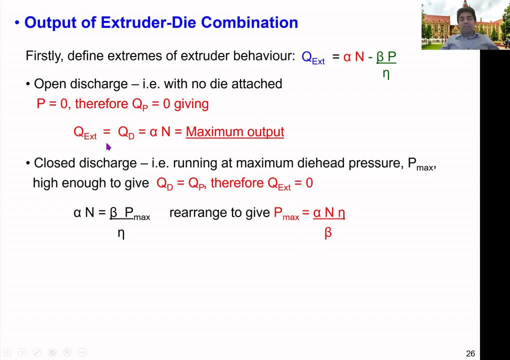 is the maximum possible diehead pressure, okay, And this is the maximum output from machine. So in this case, having the maximum possible diehead pressure means we are getting the lowest possible output from the machine. okay, As I said again. so this is indicative only, So we assume that there is no. 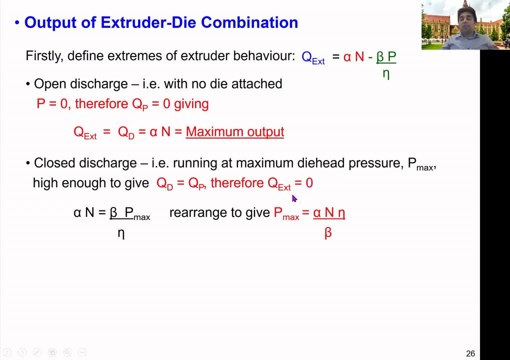 output okay, But we are not running extruders with zero output, okay. So while closing the output, So. but we can run the extruders with no material sometimes, But again it is not good, It can just damage the screw. So therefore, please don't try to run extruders without material. So 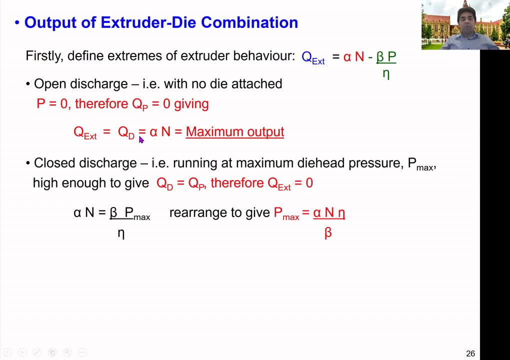 then it could create some issues as well. So that is the maximum possible diehead pressure. So here we want to just look at what is the maximum possible output. So that is the open discharge, There is no die. And then this is indicating the lowest possible output. That means 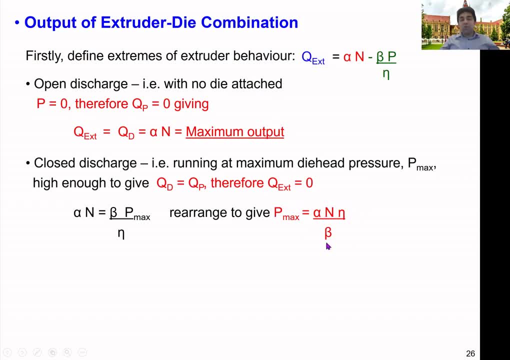 the highest possible diehead pressure. So this is how we get those: the two things: maximum output and the maximum diehead pressure. So this is the volumetric flow rate, That is, the output from an extruder, actually okay. And also we discuss an equation for the Q die or the volumetric flow rate. 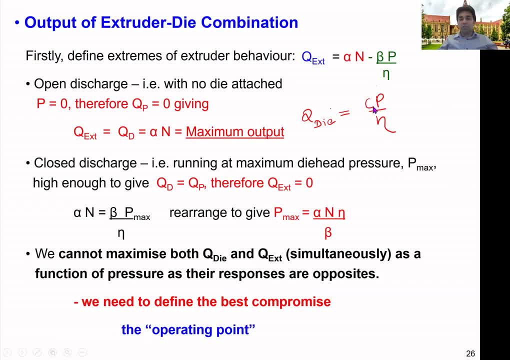 of a die as well. So it is the C a die geometry constant, and then the pressure and the eta here, or the viscosity of the material. But here it is obvious that. So we cannot maximize both Q die and Q ext simultaneously. okay, As a function of pressure, as their responses are opposites. 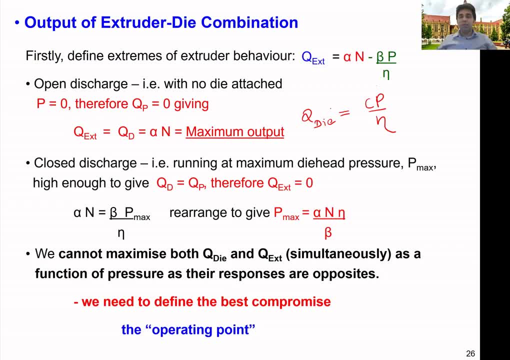 Hope it is quite clear what is happening during the extrusion process. actually The screw is turning and then material is just conveying along that and then screw is trying to push the material but die is connected at the end. So then the flow inside the die is pressure driven. So 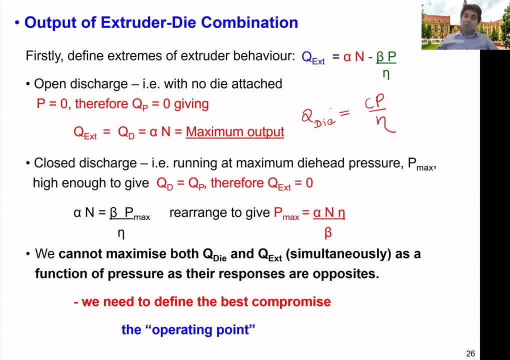 if you want to force the material through the die, so then it will create some the negative flow, which is we call the pressure flow. So therefore the Q ext and Q die, they are having some opposite responses. So therefore we have to get some the best compromise. So that means we have to select. 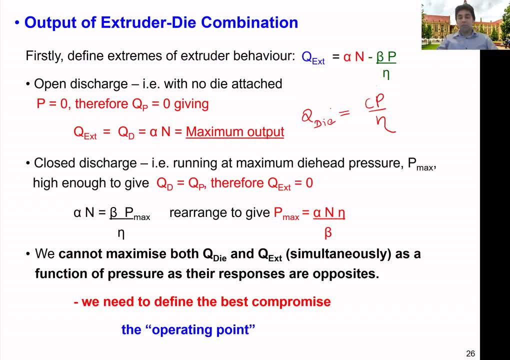 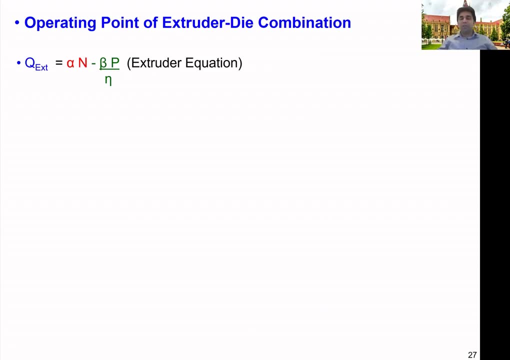 a suitable operating point for a given extruder to maximize the output or to just get the required the processing conditions to manufacture a given product. Okay, Now I just mentioned you that the extrude output and die output, they are having some opposite responses, right, Let us see how we can get an optimum operating point. Let us try to. 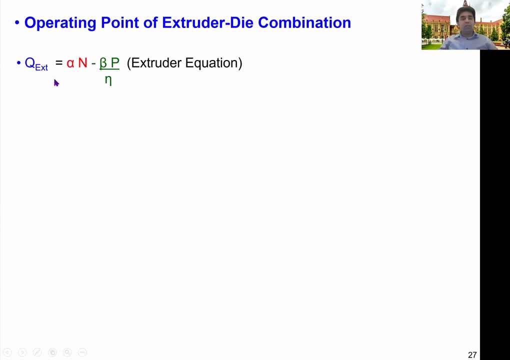 study these two equations in detail, actually. So we have the equation for the extrude output Q. ext is equal to alpha n minus beta p over eta, So we call this extrude equation. So let us try to plot these two equations using the axis, actually So in this graph. 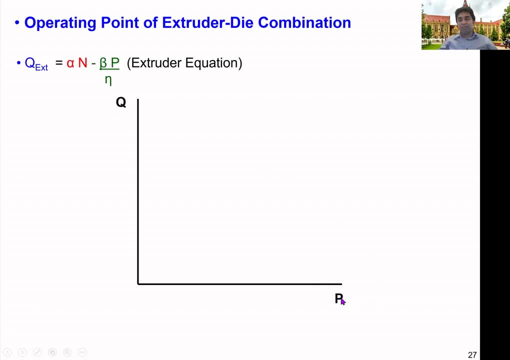 the y-axis is the Q, that is, volumetric flow rate, and then the x-axis is the p, so which is the die, head pressure. Okay, So then, if you try to just plot this equation here now, so you could assume that if there is no pressure, or the pressure is zero, or if there is no die, 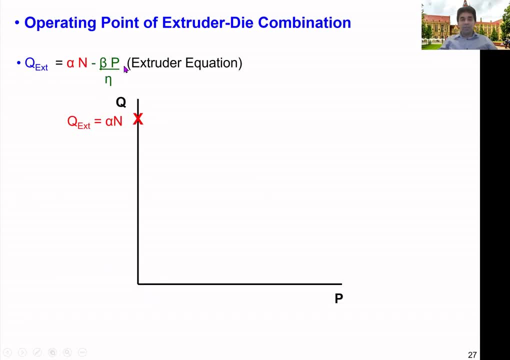 attached. so then p is going to be zero, right? That means this whole term goes to zero, So then we can have the maximum possible output. then Q ext would be alpha n, right? So then we can mark it here, So without a die attached. 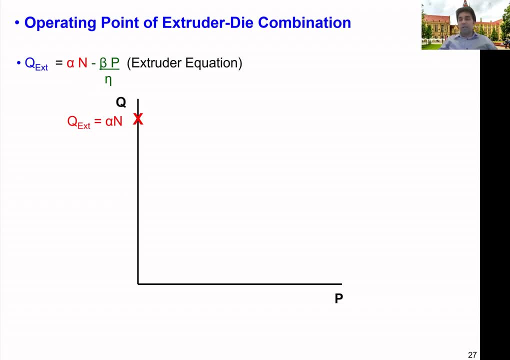 so we can have the maximum possible output from an extruder, but it is not useful because we can't force the material through a die, so then we can have only molten material. So then the next situation that I am going to look at is the Q ext is equal to zero, so there is no output. 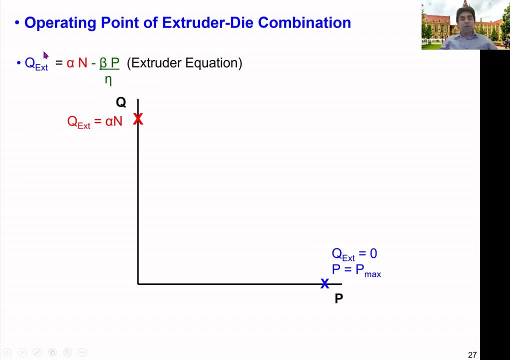 If there is no output, then we can move this term into the other side, or that means alpha n should equal to beta p over eta. so that is what we discussed before. that is the closed discharge and this is the open discharge. okay, so for the closed discharge we can get the maximum possible. 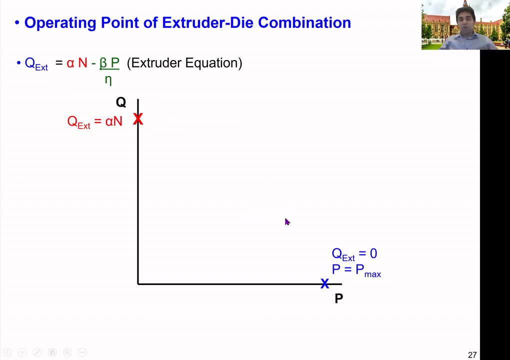 pressure. so in that situation we can assume that there is no output from the extruder. so then we can draw the extruder equation within this graph. okay, so we can just draw it in this way, now, right. so then this is the open discharge- maximum possible output- and then here the closed discharge. 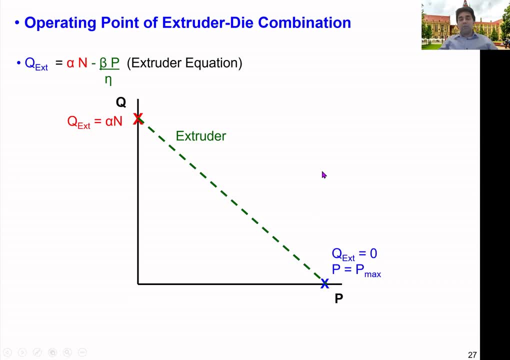 there is no output but the maximum possible diet pressure. so then let's try to add the, add the, the die equation into this one. now, okay, so the die equation we discussed before, which is c, p over eta, cb in a geometry related constant, so it is really simple one to just 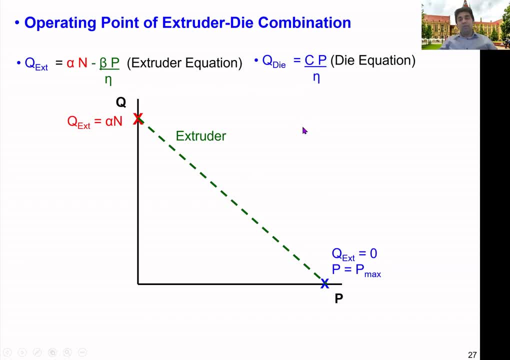 the, the draw here in this axis, actually. okay, so, initially. so the p equals to zero means so then there is no output. okay, so then it should be starting from here. okay, so then, uh, the p equal zero means the q die is equal to zero, the output from the die is zero. okay, so that's then we have. 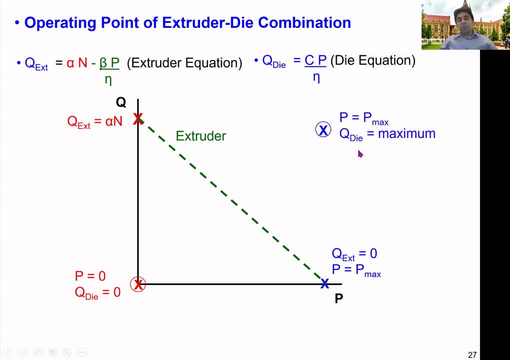 to start from there and then the for the maximum pressure so we can get the maximum output or the best possible for within the die. okay, so that is obvious. so then we can push the material to the die quite easily as long as the pressure is high. okay, so with the maximum possible pressure we can. 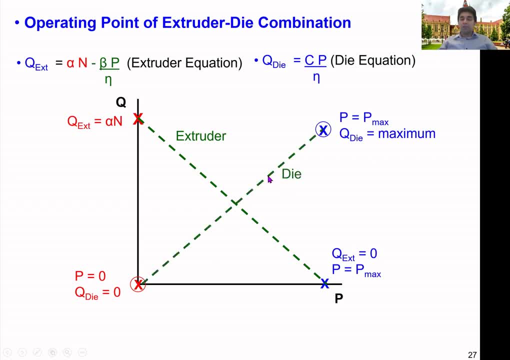 get the maximum output or the maximum flow through a die. so then we can get the die equation just the drawn in this way now. so this is what i mentioned before, that. so the extrude output, q, e, x, d and the die output, they are having opposite responses, okay. so therefore they are just the 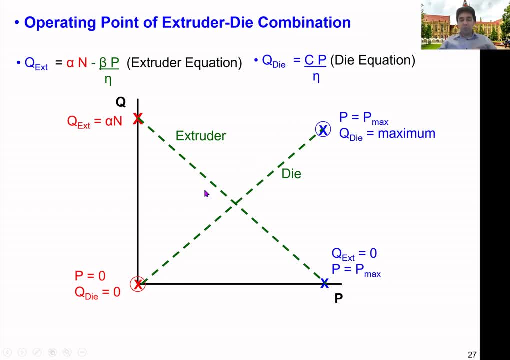 opposite to each other. so then, so we can just pick the operating point right. of course, here now we could see that. so this is the best possible operating point. okay, for the optimum performance. right now, the question is that: is this the best possible operating point that we can run? 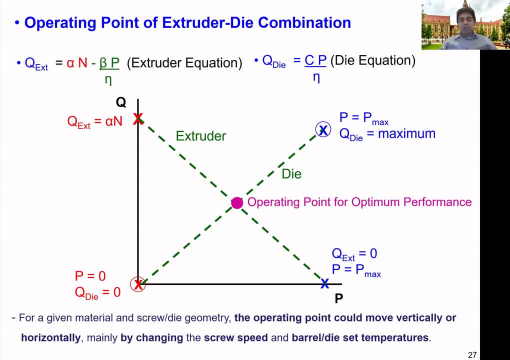 and extrude it okay. so obviously, if you don't consider any other factors, okay, this could be the best possible operating point, but in the industry so we have to consider several factors. we have to consider energy consumption, the required output, okay. the quality of the belt: okay, there are several other. 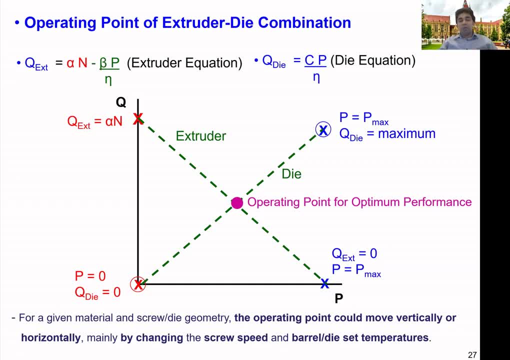 factors to be considered now. so then the, for example, if you just want to consider the energy consumption, normally, if we can run the process at the highest possible screw speed, the specific energy consumption is the best. okay, okay, higher the speed, the specific energy consumption is the best. the specific energy consumption means the energy. 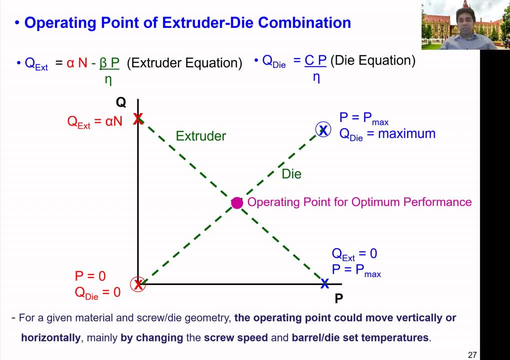 required to produce the unit amount of the molten material, let's say to the energy required to produce one kilogram of material, for example. so then, higher the speed, so the better the energy. energy efficiency right. but on the other way around, higher the speed means that could be high level of thermal. 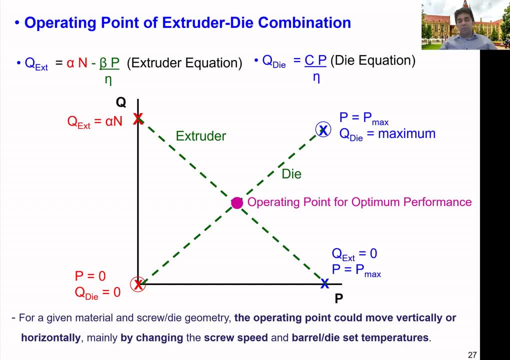 fluctuations as well, right so, therefore? so then, if you want to get the the best possible efficiency in terms of energy, so we have to run the process at a highest possible speed and then and? but it could create some thermal fluctuations, okay, so therefore we have some issue then, and also for 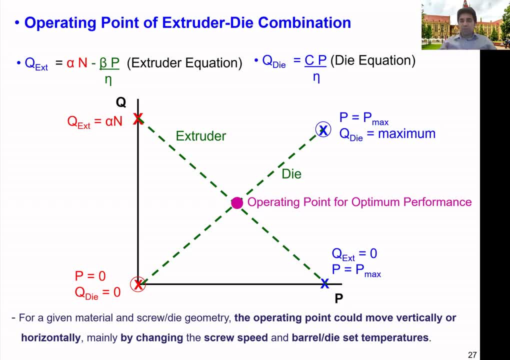 some given products, we have to maintain some certain output from the machine. for example, let's say, for a given product we need to maintain the 10 kilograms per minute, okay, so therefore, we have to maintain the certain squeeze speed to achieve that output. so so, therefore, the selecting, 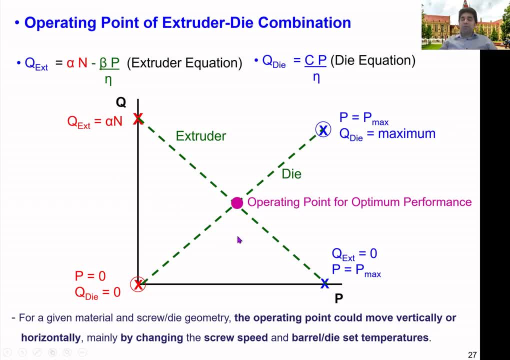 the best possible operating condition is really complicated. actually, if you consider the current industrial practice is that for most of the extruders they are not well developed with the current or the modern technology. so most of the processors they still use the screw speed and the barrel die, set temperatures as the main process control control parameters. okay, if you. 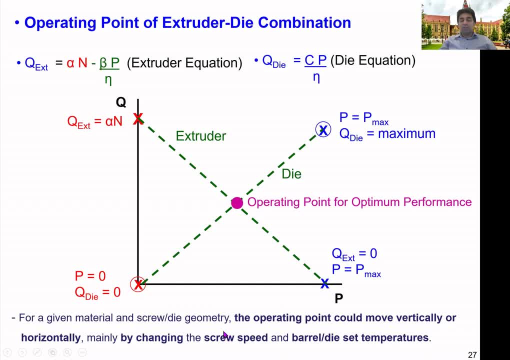 want to change anything index in an extrusion process industry. what they normally do is we just change the squeeze speed and then also they can change the barrel set temperatures. so those are the two main controllable parameters for a given machine in the current industry by changing the squeeze. 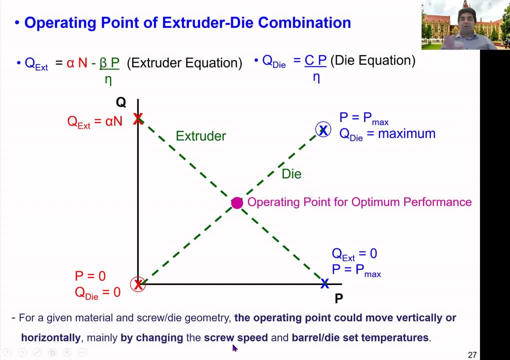 speed. so everything will change. okay, that means i i mean output will change, the pressure generation will change and also frictional and viscosity dissipation. everything will change. where temperature will change, viscosity of the material change. so these parameters are complexly coupled to each other, right? so by changing these parameters now, uh, the we can just try to influence. 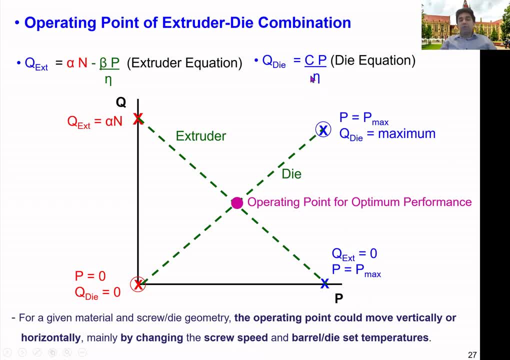 the other parameters. for example, let's say we want to just change the viscosity of the material for some reason. okay, so then we can try by changing the squeeze speed. okay. so therefore, this viscosity, melt pressure or melt temperature, they are not some parameters that we can control directly. 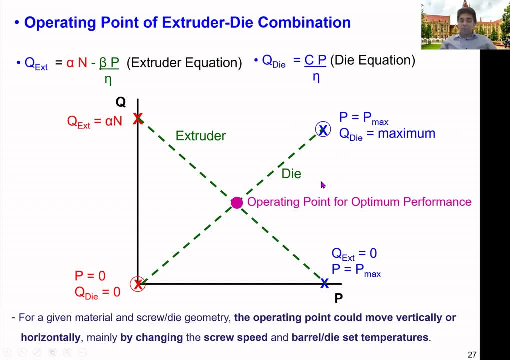 so we can control them indirectly. the main controllable parameters in direct parameters means the squeeze speed and barrel dioxide temperatures. so by controlling these two, okay, or by changing these two, we can just try to move this operating point, uh the horizontally over to get the the desired output from an extruder. okay, by considering the cost factors, time. 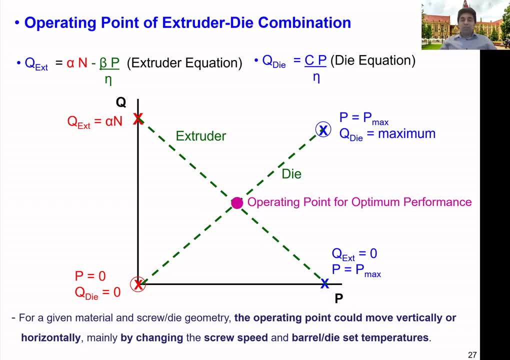 consumption- energy consumption, labor or the other- the quality of the melt- and then, based on that, you can try to place an extrusion process in the best possible- uh, the the best possible operating point. okay, so possibly it could be. you should try to just get this line to be like this and then